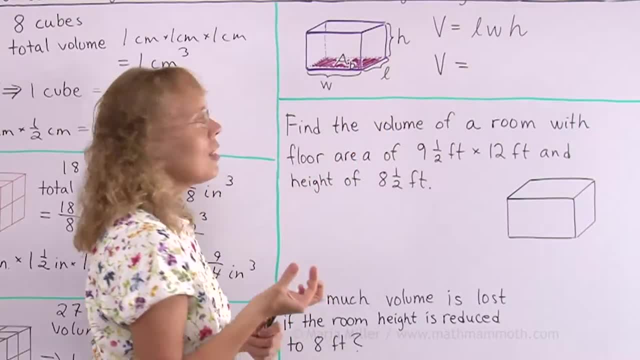 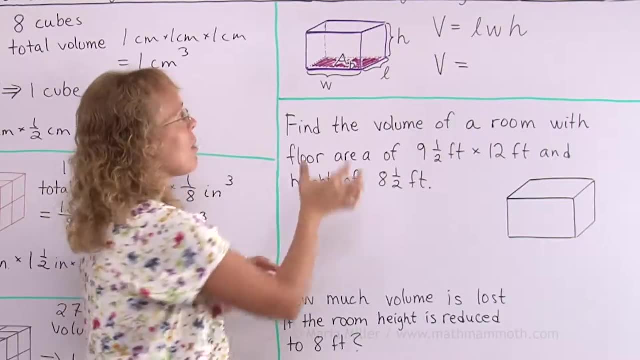 whichever you want to think about, these two dimensions multiplied together actually gives you the area of the bottom right, The area of the bottom. The bottom is a rectangle, so you find its area by multiplying these two. So I can write another form of the same. 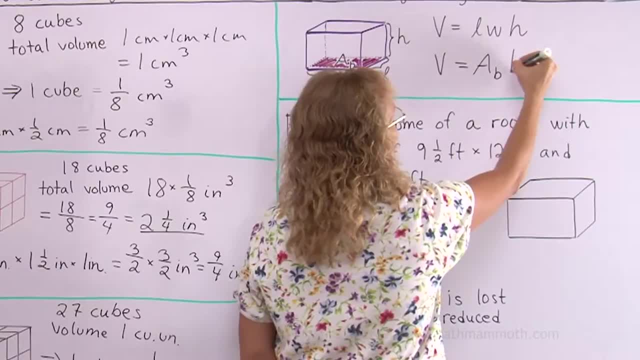 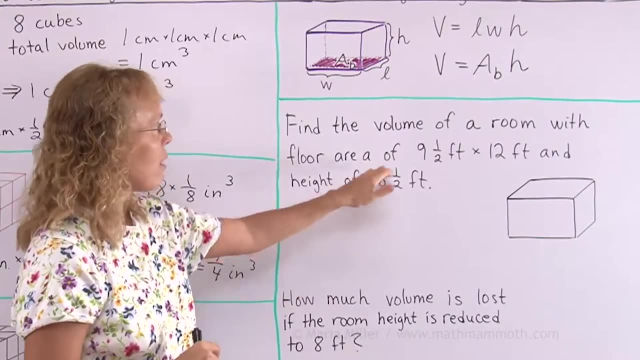 formula You can take. these two are the same as the area of the bottom times the area height. Alright, let's solve this problem now. Find the volume of a room with floor area of nine and a half feet times 12 feet, and then height of eight and a half. 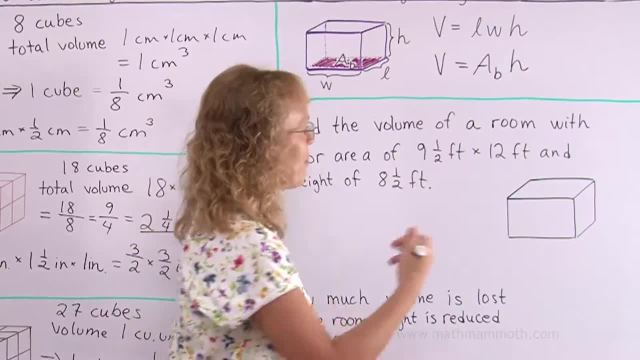 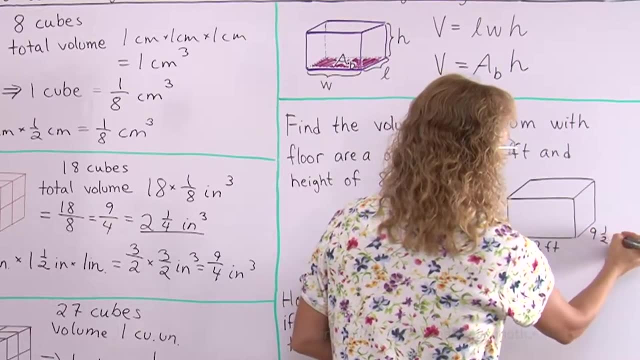 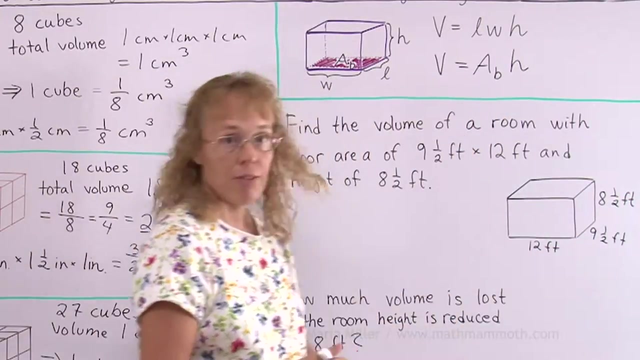 feet. So here we have our fractions. Okay, if I mark here in the picture, let's say this is 12 feet, this way is nine and a half feet and the height is eight and a half feet. Let me first multiply to find the floor area here 12 feet times nine. 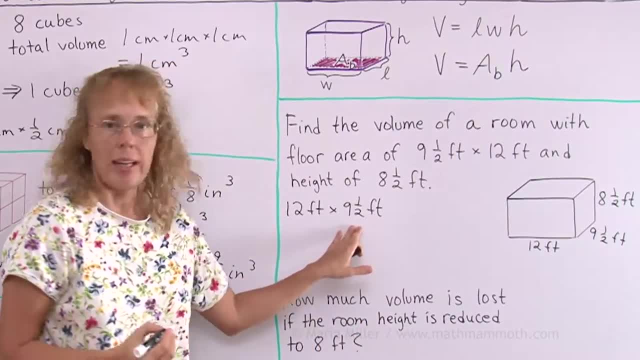 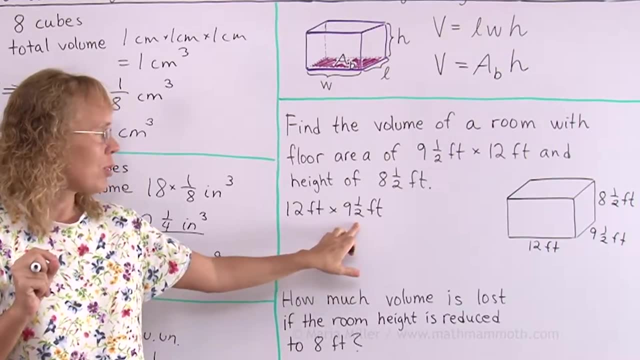 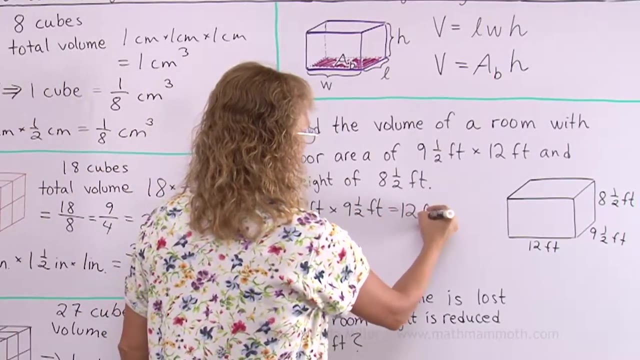 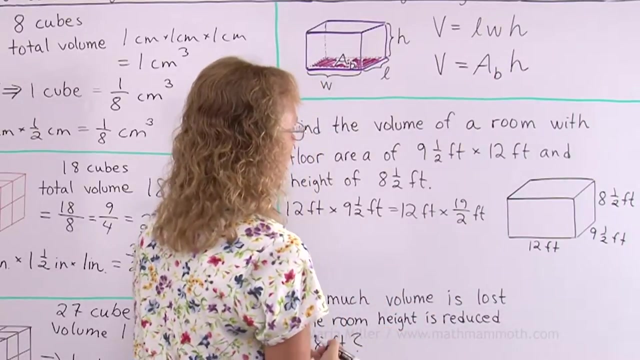 and a half feet. Here's a mixed number, So to multiply with it, you will convert that into a fraction. first, Nine times two is eighteen plus one is nineteen, So we get 12 feet times 19 over 2 feet. okay, and now here, in this expression, the 12 times 19, and then 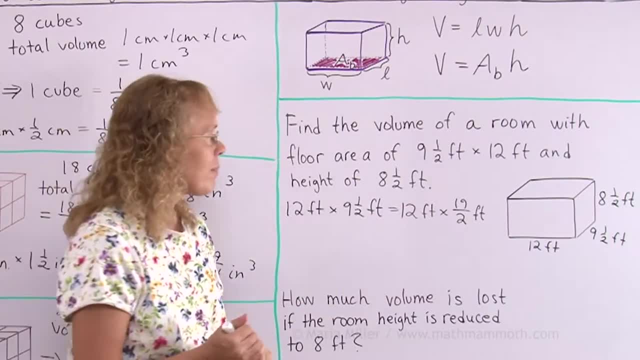 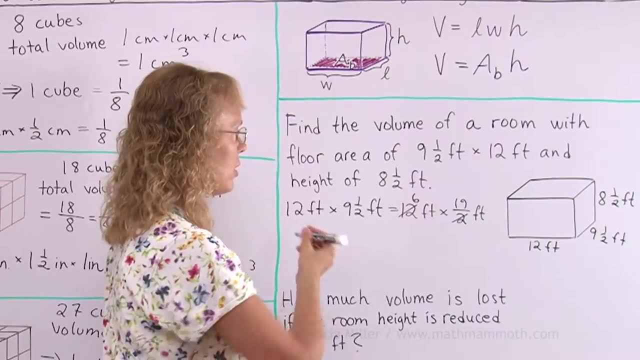 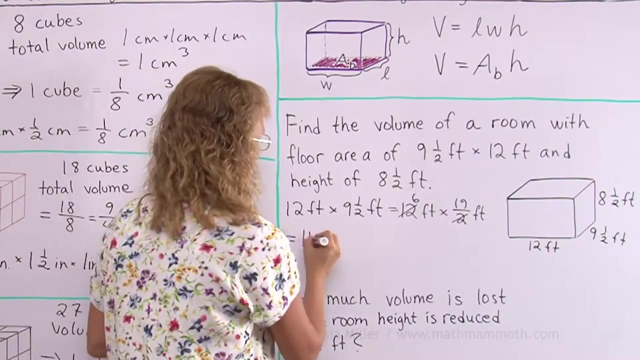 that's divided by 2. I can simplify just a little bit, because instead of dividing by 2 I can just cancel that and in the beginning multiply by 6. so it's 6 times 19, and that is 60. plus 54, it's 114, and our unit here is square feet. that's the 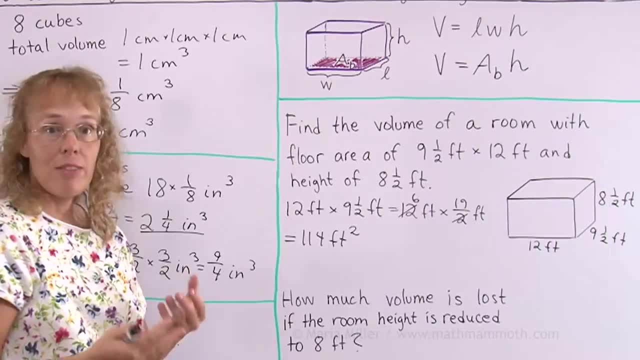 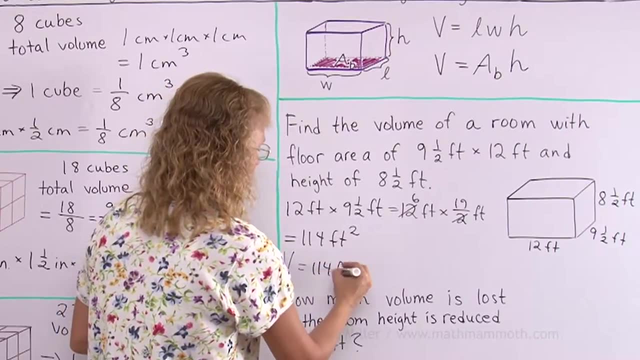 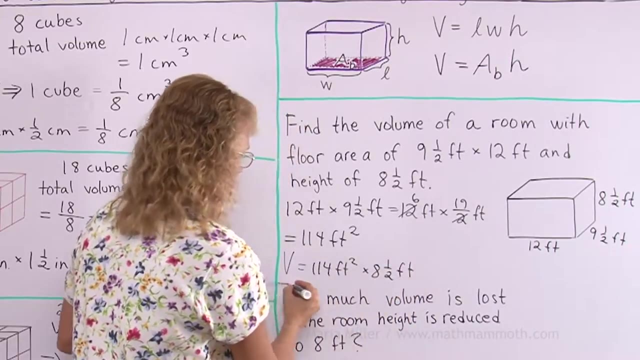 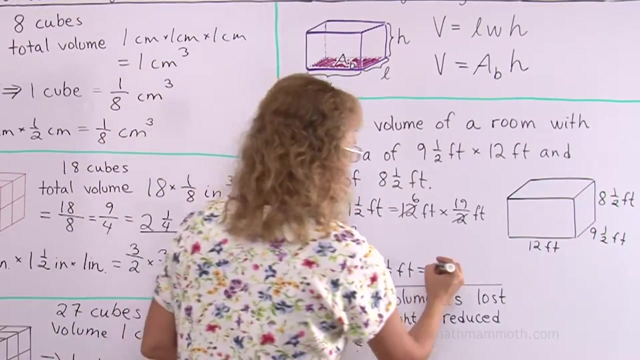 area of the floor. okay, and now to find the volume, I will take this and multiply that times the height: okay, V for volume would be 114 square feet times the height- eight and a half- okay, again eight and a half needs to change into a fraction. we get 17 over 2. so 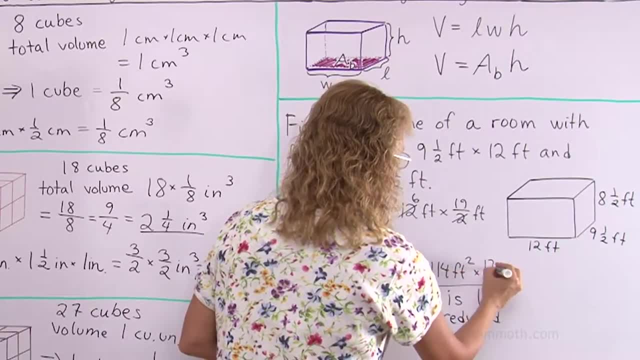 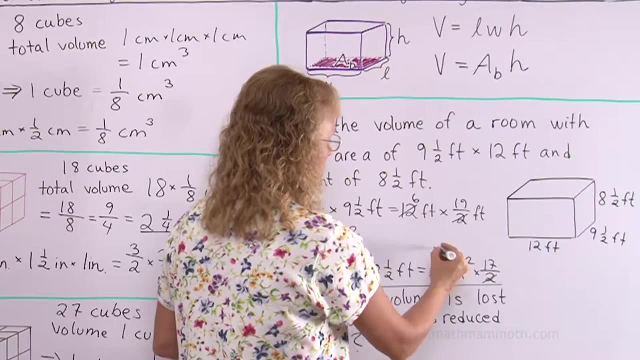 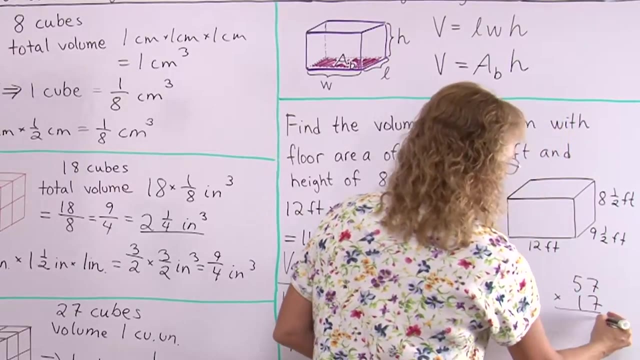 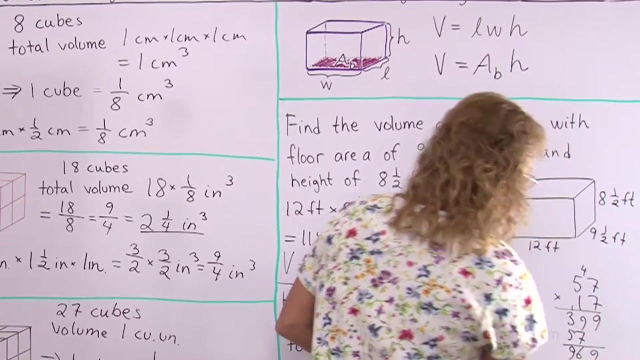 there's 114 square feet times 17 over 2. here I will simplify again: take just half of 114, which is 57, and now we will multiply 57 times 17. that's 49 and 39,, 7 and 5. okay. 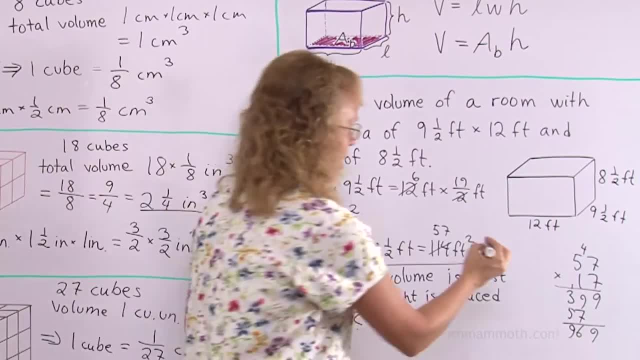 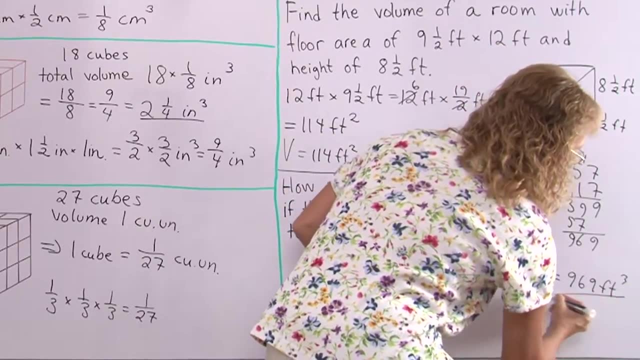 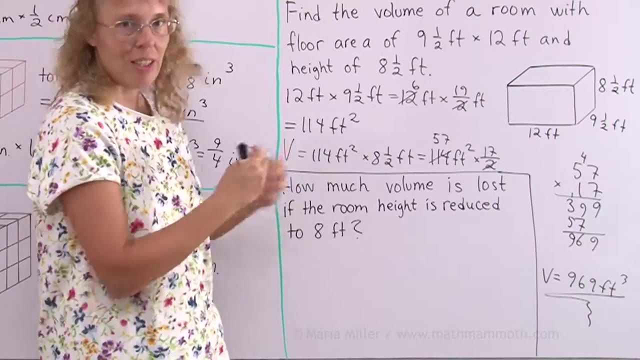 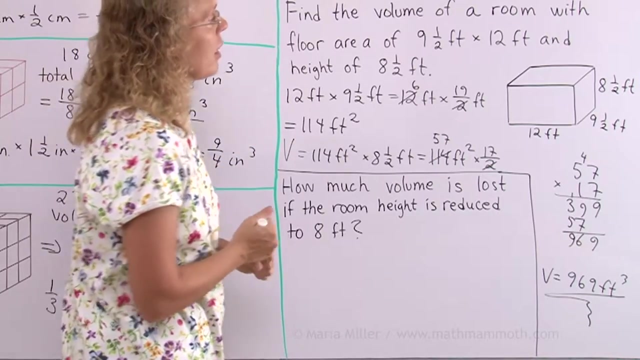 so I'm running out of space, okay, but the total volume here is not nine hundred and 69 cubic feet, okay, so we didn't get a fraction as a result, because they canceled out and stuff. now how much volume is lost if the room height is reduced to eight feet of the? 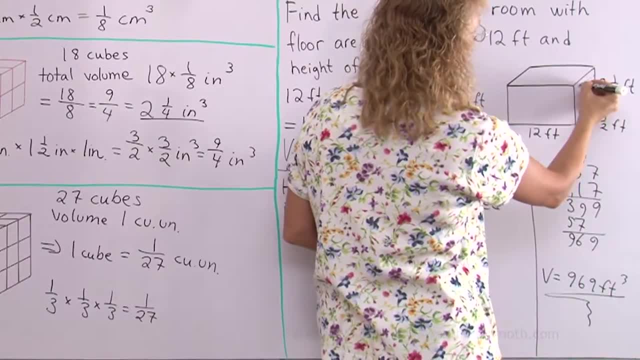 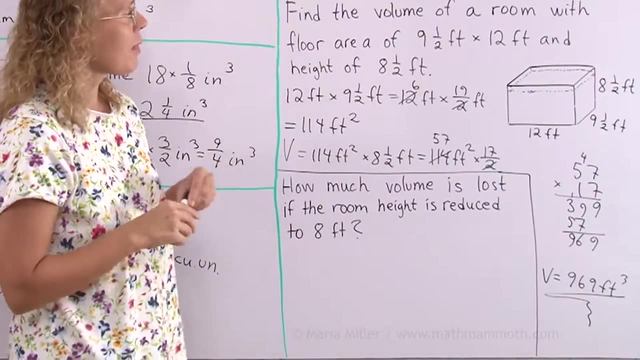 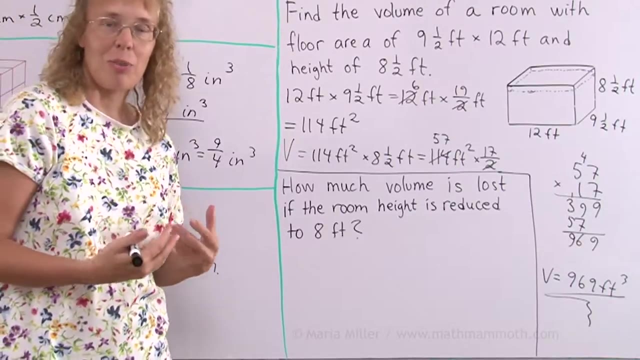 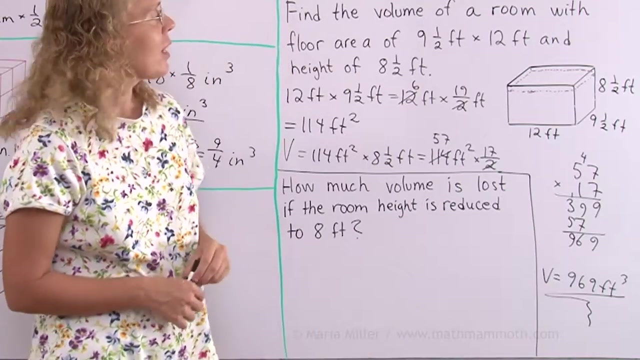 room height is reduced to eight feet, go somewhere here. how much volume is lost then? You could solve this in two different ways. You could solve first: how much is the new volume, how much is the volume if you use 8 as a height, and then subtract this and your new result? Or you can just think: 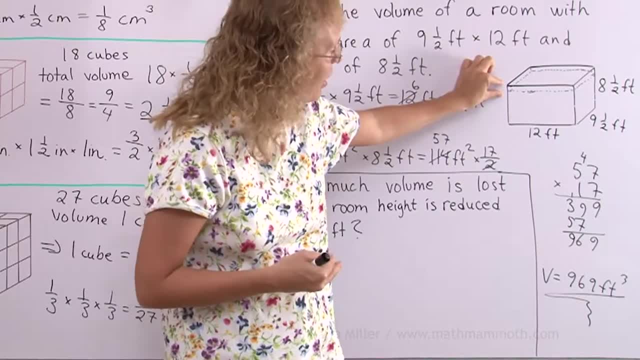 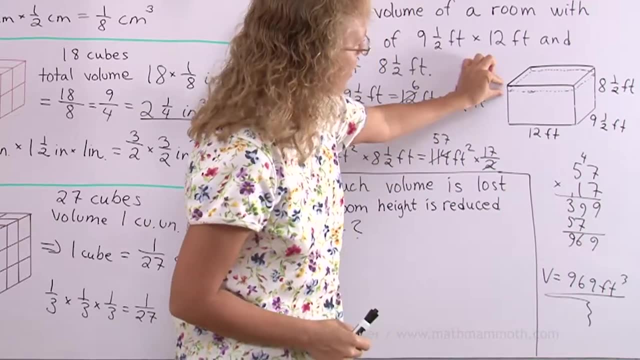 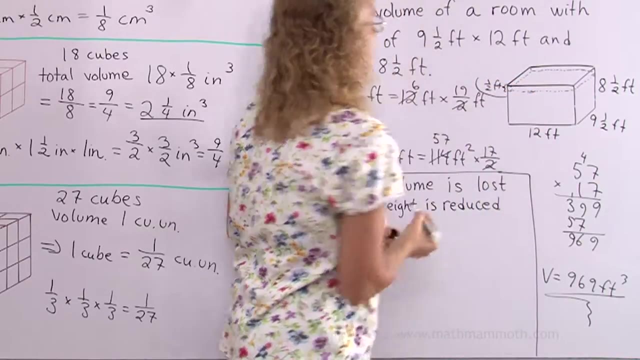 of this part that will be taken off the top of the room, so to speak, because it is a box too. It is a box shape, or a rectangular prism here too, and its height is half a foot right, This one, Because it is reduced by half a foot over here. So I can just calculate. 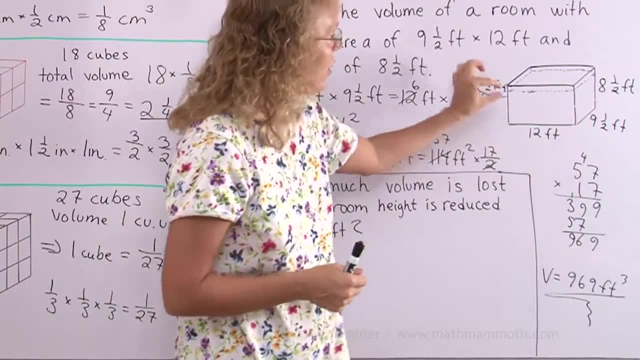 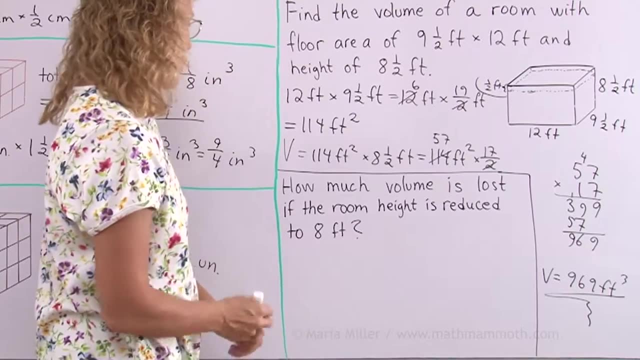 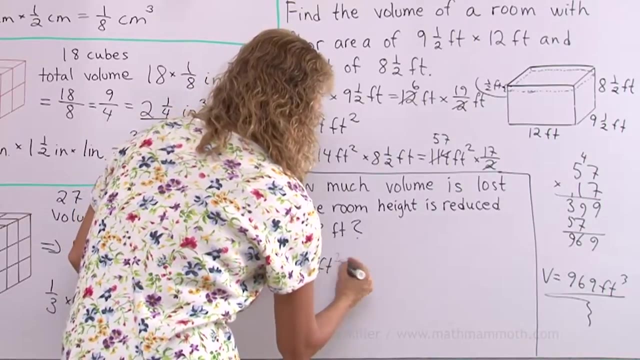 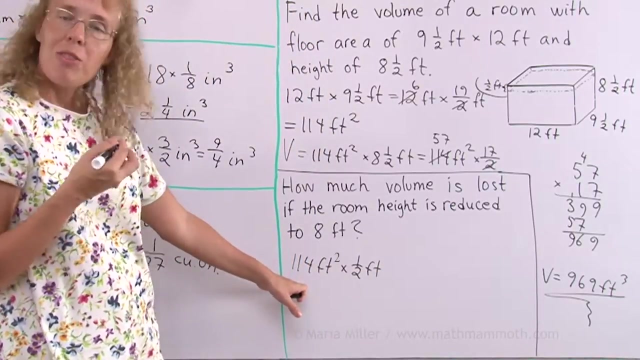 the volume of a rectangular prism with the same floor area and height of half foot, and that's how much the volume is reduced. So I can take the floor area which was calculated here. This is 14 times the height that it is reduced by to half the foot. So this is 114 times. 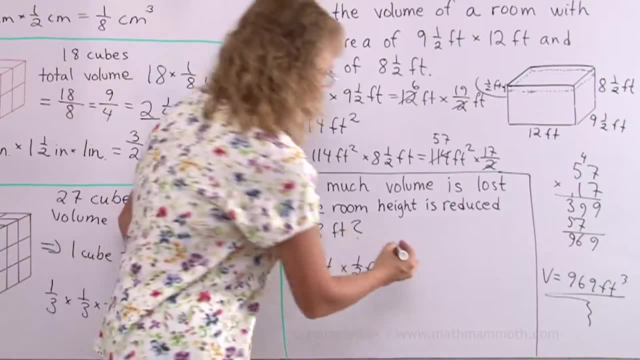 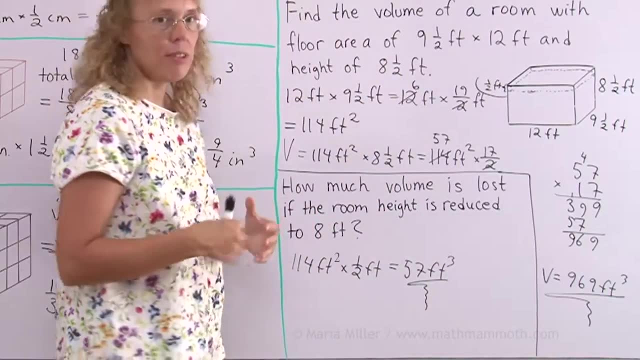 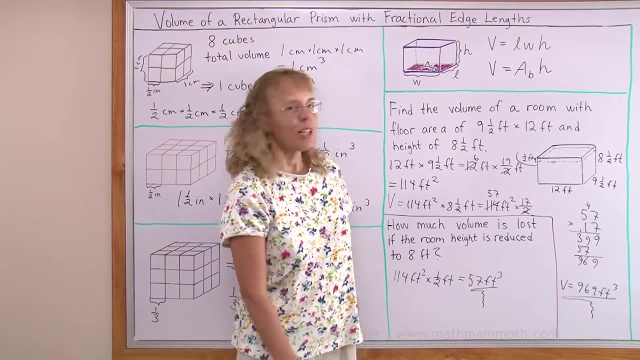 half Or half of 114. So that is 57 and the answer is again in cubic feet. That's how much the volume would be reduced, And the new volume, of course, would be that number minus 57 cubic feet. Okay, Alright, we are all done with this, And I hope this was helpful. Thank you very much. Thank you very much.